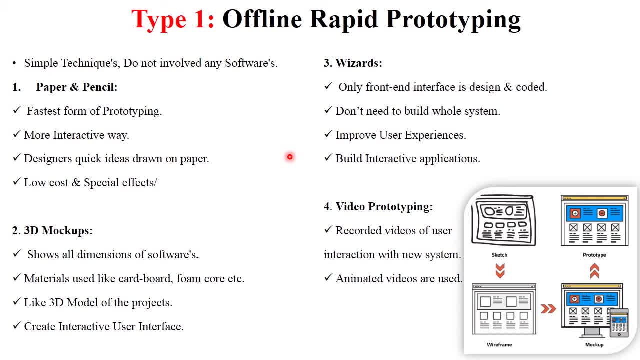 While implementation of particular project or in software development life cycle, the designer- designers- has the one, one of the most important stack holder in complete software development life cycle. So designer use all those prototyping techniques to develop a prototype. 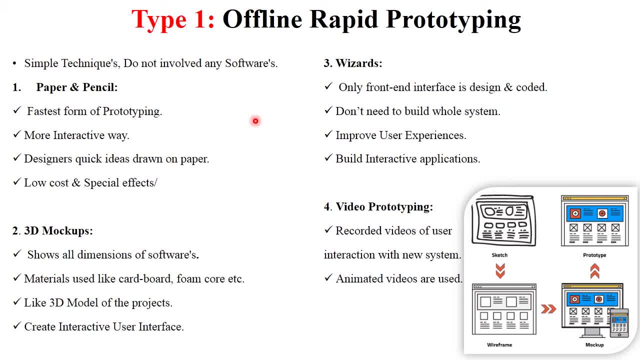 That is, online, offline. this technique for development of particular project. So if you design a particular software properly or as per the requirement of the customers, then only programmer or developer implement those project or those software more effectively. okay, 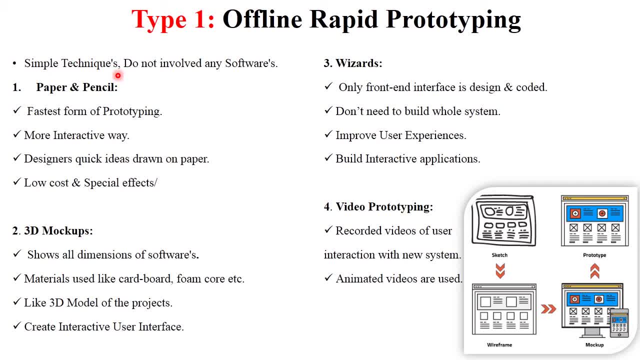 So design is one of the most important part. So offline rapid prototyping is one of the simple technique. do not involve any software. This technique includes paper and pencil approach, 3D mockups, results and video prototyping. 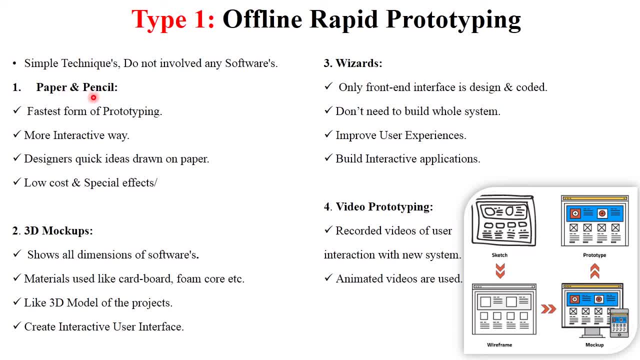 So first approach is paper and pencil. So by using paper and pencil you should draw a design, or you should draw your ideas on paper How exactly particular software, particular application will be built. So paper and pencil is fastest form of prototyping and it is the most interactive way. 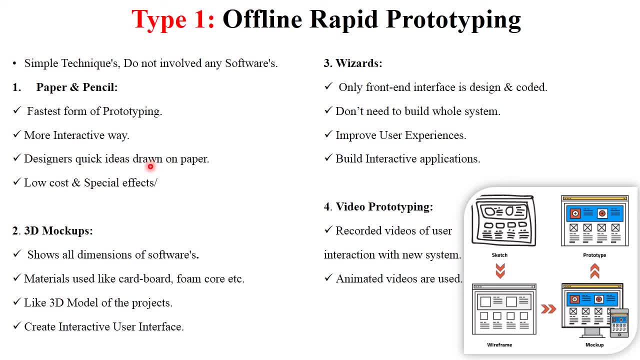 Designers quick ideas drawn on the paper, and paper and pencil has low cost and special effects right. So paper and pencil is one of the most easy approach. Another one is 3D mockups. it shows all dimensions of software. 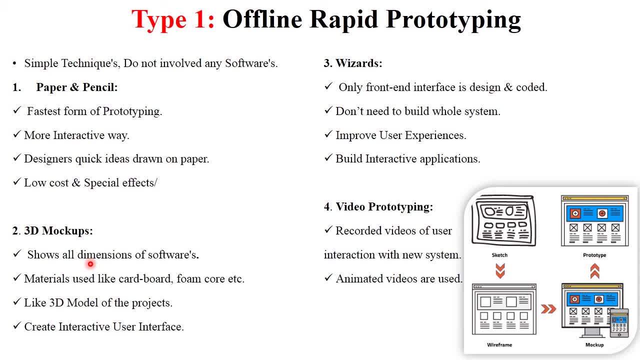 By using all dimensions or by using 3D approach. you should analyze how exactly the particular system work. It use different types of materials like cardboard, foam, core, etc. Generally, 3D mockups are very easy to use. 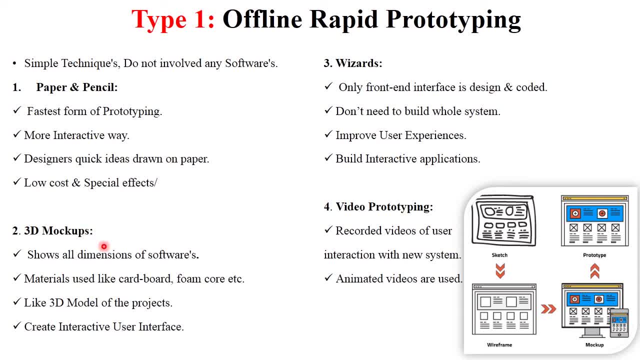 So paper and pencil is one of the most easy approach. So paper and pencil is one of the most easy approach In 3D mockups, this prototype technique used in architectural field, like 3D models of that particular project, and which is create a interactive user interface right. 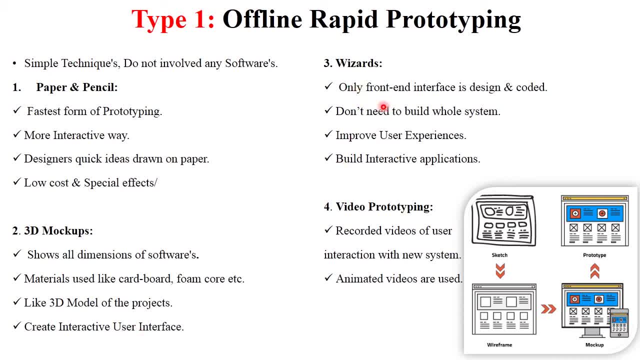 The next approach is wizards. Wizards means only front end interface of the design or coded. ok, It don't need to build whole system. Suppose, if you open a login screen, you should attract with that particular approach, a particular screen. 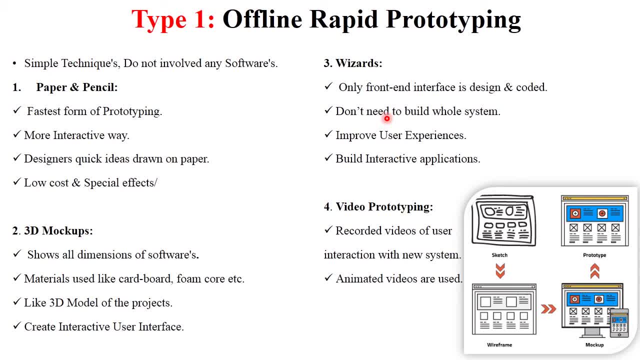 Right that you don't know about how exactly it will be coded. Right, wizard means just front end approach. Suppose if you, if you should visit a particular website, right? So website is a front end interface. It is called as wizard. 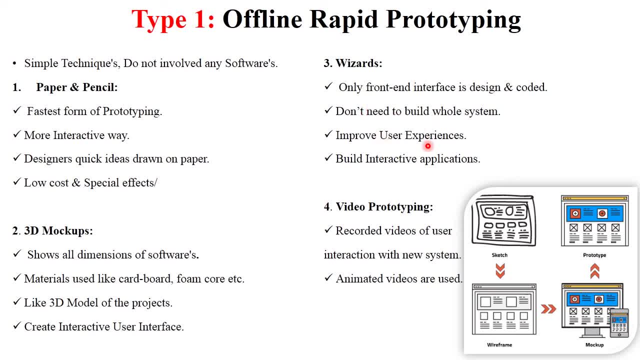 Don't need to build whole system. It improves the user experience and build the interactive applications, Right, Because user mostly attracted with the front interface only, Right, Right. The next one is video prototyping. Video prototyping means to record a video of user interaction with new system and also some animated videos also used. Okay, So you should make a particular video or animated video how your project will be work, how your system will be developed like this, Right. 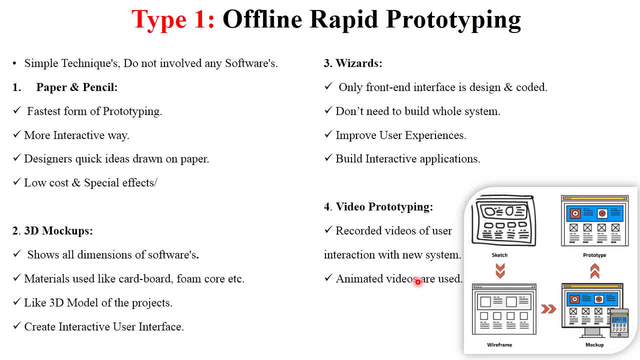 So these are the offline rapid prototyping techniques. You must use this technique before implementation of particular project. See in this diagram. first you should just sketch a particular design. Right After that there will be a wireframes, then mock and then prototype. 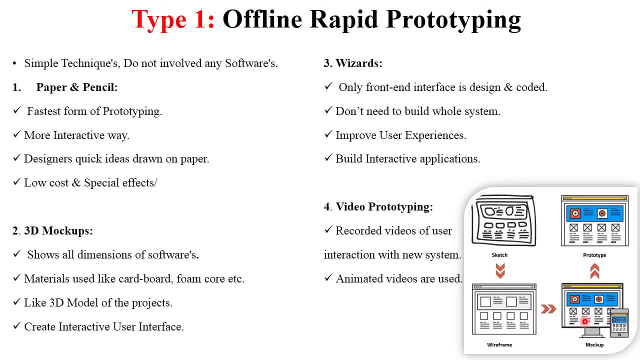 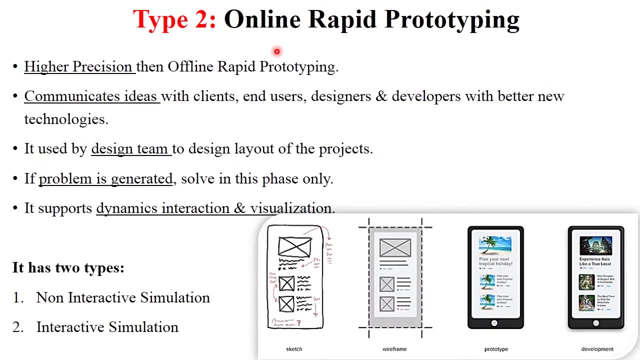 So wireframes and mockups use the different types of software, sometimes Right, And after that your complete prototype is developed And this prototype is given to the user Developer or the programmer for implementation purpose Right Next, The next and second type of rapid prototyping is online. So online rapid prototyping has higher precision than offline rapid prototyping. 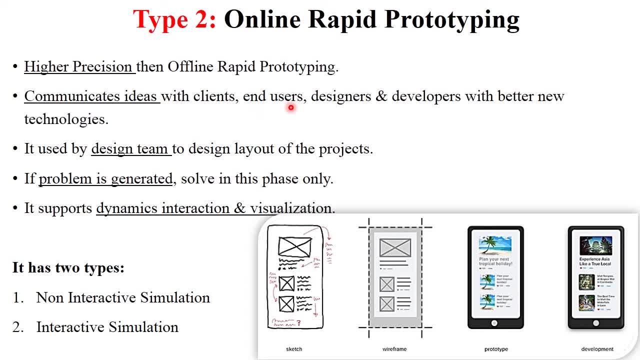 Because it communicates ideas with clients, end users, designers and developers. with better new technology Right. It used by design team to design layouts of project. Okay Next Online rapid prototyping. you should use different softwares, frameworks, different types of libraries for development or design a particular project. 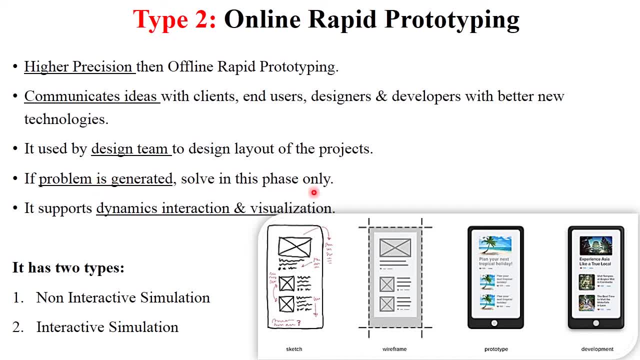 And if problem is generated, so solve in this phase only. While design a particular software, there are some problem will be generated. You should analyze those problem. Suppose you should design a particular way, then which type of problem is generated? So there are many options are given. 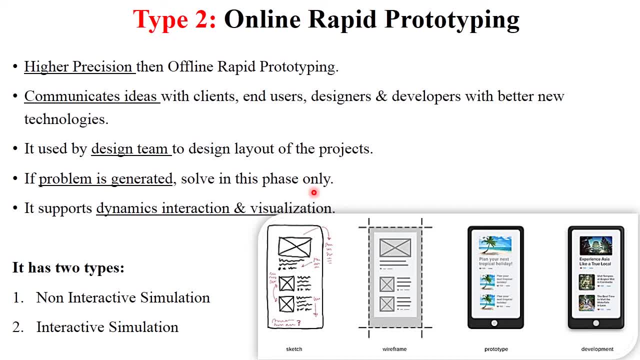 Okay, So after design a perfectly design a particular software, then only you should implement a project. So it supports dynamic interaction and visualization Right Online. rapid prototyping has two ways: Non-interactive simulation and interactive simulation. So let's see what is meant by this kinds of simulation. 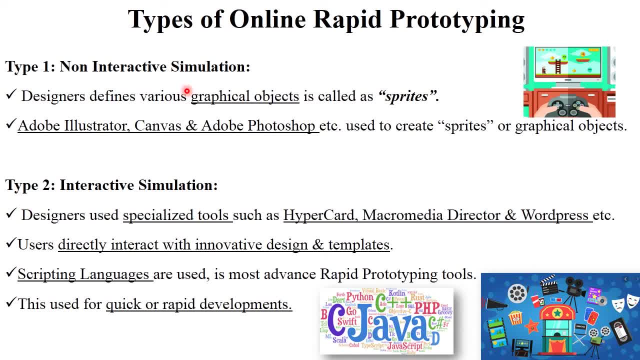 Next. So there are mainly two types of online rapid prototyping. The first one is non-interactive simulation. The second is interactive simulation. It design as, define a various graphical objects. It's called as sprites. Okay, So by using different softwares like Adobe Illustrator, Canva, Adobe Photoshop, 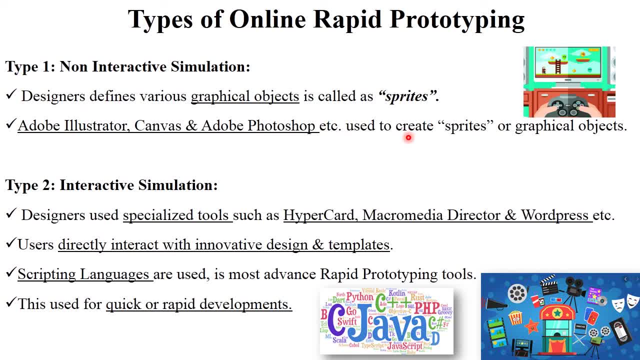 By using this objects or by using this software, you should create a particular graphical object, And this graphical object is called as sprites Right. So you should use this kind of softwares for designing a particular project or application. And a next type is interactive simulation. 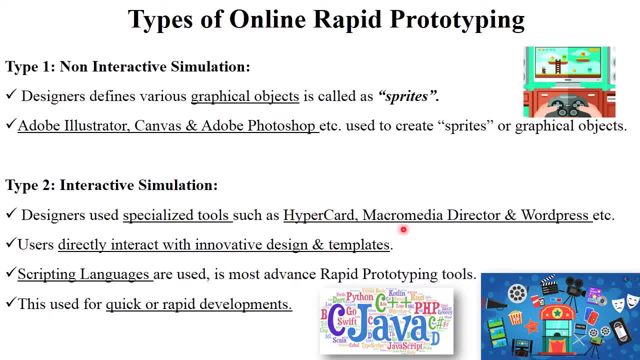 Designers use a specialized tool such as HyperCAD, then Macromedia Director, Wordcase, for designing a website like this, So user directly interact with innovative designs and templates through this. There are different free templates and also some cost templates are available. 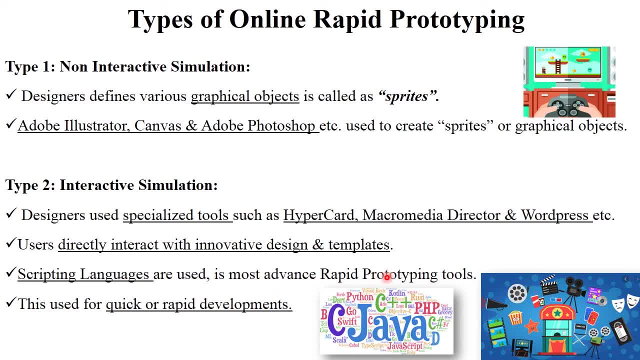 Scripting language are used is most advanced rapid prototyping tools. You should use different types of programming language for development purpose as well. Okay, this used for quick and rapid development. So in non-interactive simulation it includes only designer part. 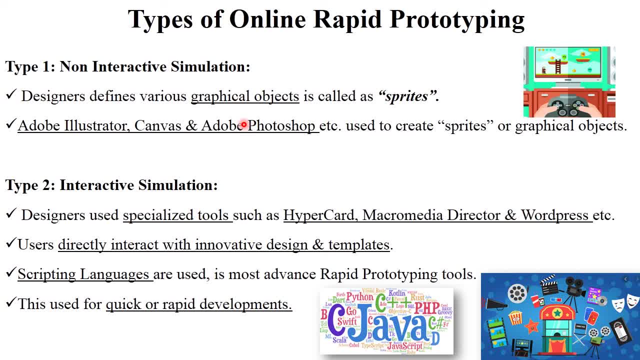 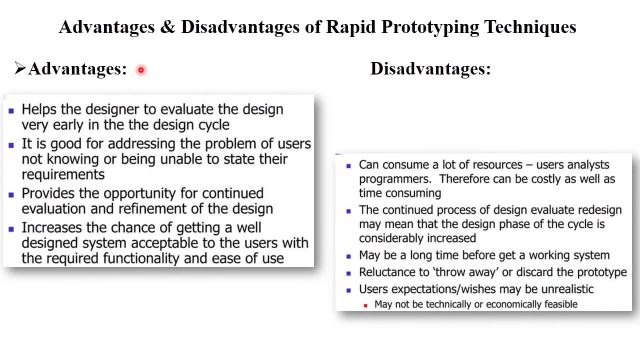 By using software, you design a particular application And in interactive simulation you should use design as well as implementation. part Right, so this: all techniques is used because of quick or rapid developments. Clear next. Now what are the advantages and disadvantages of rapid prototyping techniques? 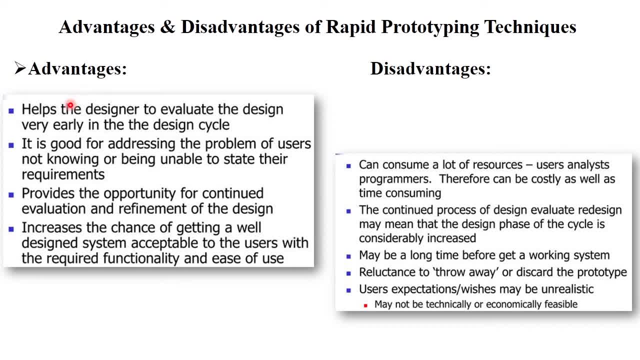 So the main advantages of rapid prototyping technique is: it helps the designer to evaluate the design very early in the design cycle. Right, it is good for addressing the problem of users not knowing or being unable to state their requirements. This as per the exact requirements of the customers or the users. you should design a software.